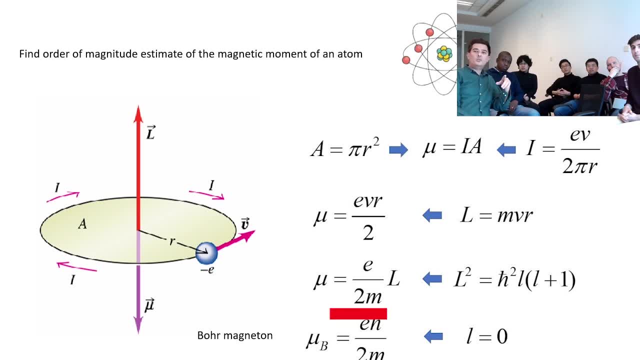 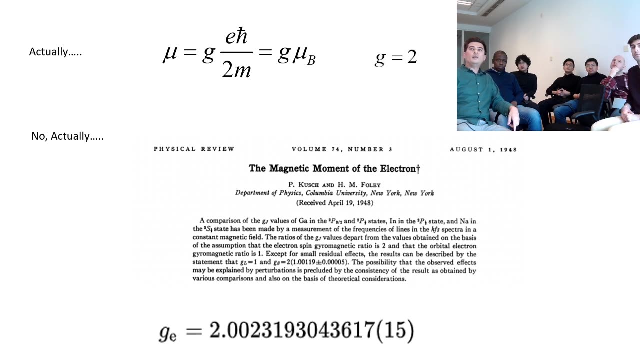 change to angular momentum and that introduces this factor of E h bar, and this is what it would be for, like you know, like a classical orbiting electron, If you actually do a quantum mechanical calculation, then it is not actually equal to E h bar over 2 m. There's this factor of this gyromagnetic ratio which is, you know, basically. you can see that. you know, this calculation is just the order of magnitude kind of estimate. So if you do a real quantum mechanical calculation then it turns out to be two. but if you actually do an even more accurate measurement then it turns out to be something a little bit away from two, right? So this was first done for the electron in like 1948. 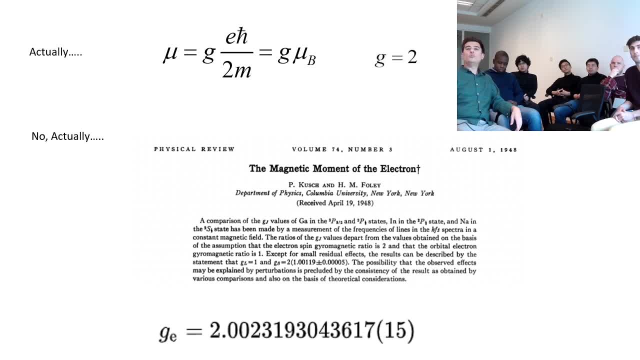 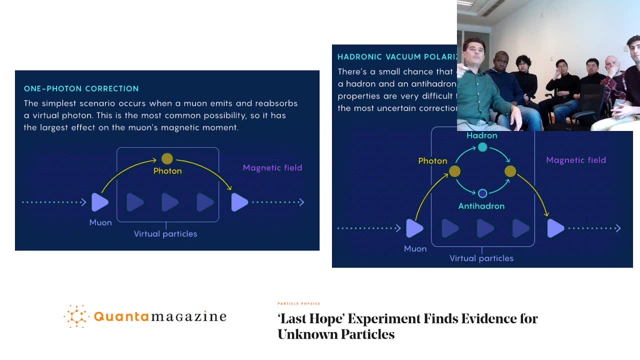 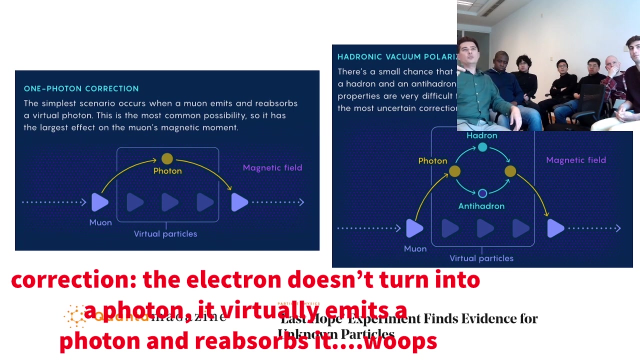 and then they found that it's, you know, a little bit above two. and why is it above two? It's basically because there are these so-called quantum fluctuations, So an electron has some kind of probability that it can turn into a photon and then come back into an electron. So that's basically. this is called the one photon correction. 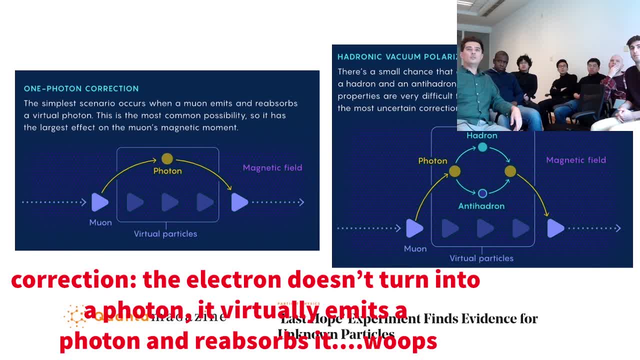 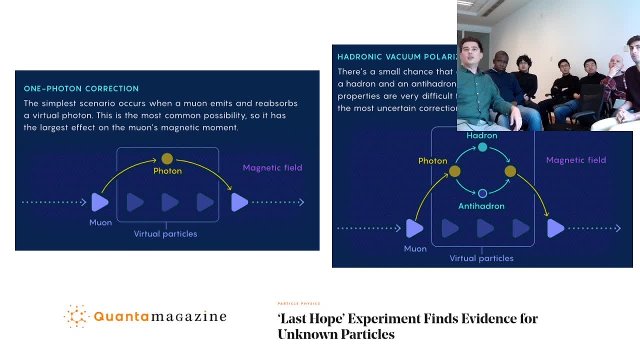 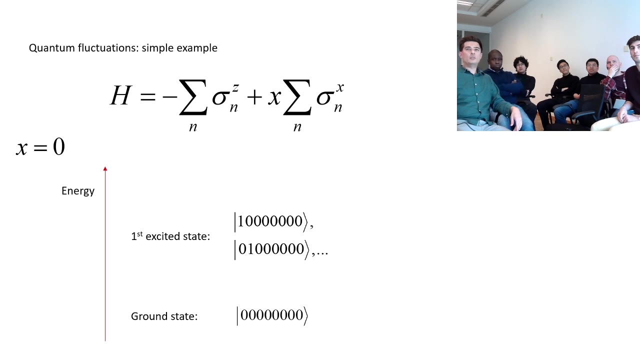 and Schwinger was the guy that originally found or explained this phenomenon- But actually for the muon there's like all kinds of other effects, like the photon can turn into some other particles, like these hadrons, and this can give like further corrections. Just to give you a bit of a simple example of what it basically means is to have quantum fluctuations. 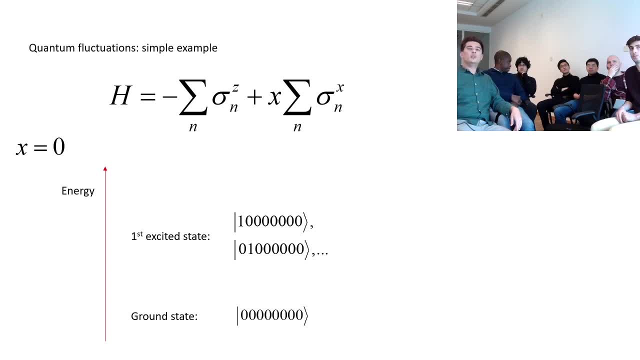 So imagine you have this like spin model where, say, all the spins are down in a particular chain and then you have some small term which is, like you know, like a perturbation on that right. Then if you diagonalize like the sigma z part of this, then you'll get like a ground state which is: 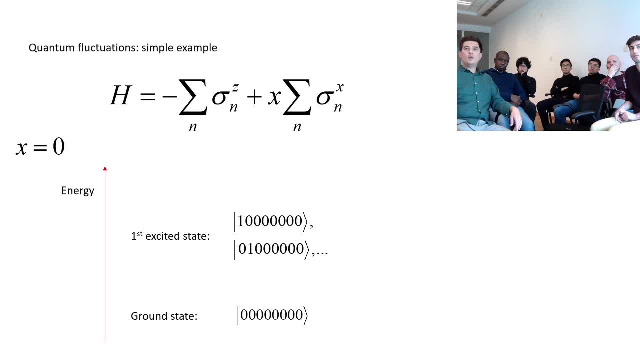 like all spins in the zero state, and then if you include the x, then you'll have a perturbation of this extra term, right? So what you call all this extra stuff there that you see, that's a superposition of the on top of the stuff that you would otherwise have. you know this is. 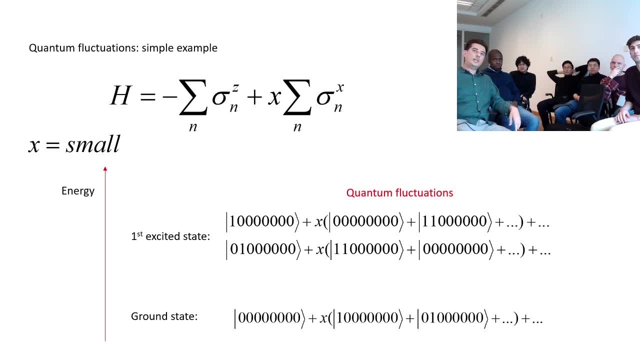 basically called quantum fluctuations, Basically. in this case it's just a more complicated version of that, but you have, you know, small terms which basically take you away from the state which you would, you know, ordinarily think. So when you say vacuum, it's not really the state where there's. 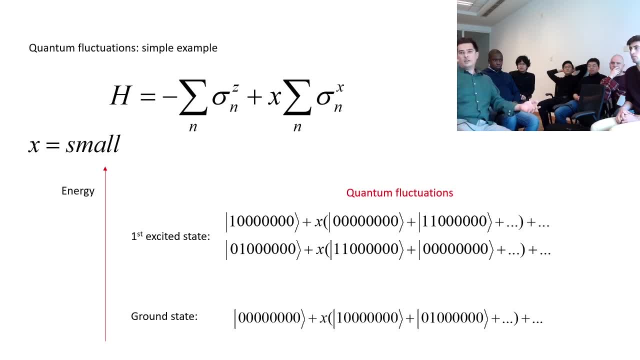 nothing actually there's. there's nothing in it, Like some other extra states which are in a superposition on top of that, and that gives so-called quantum fluctuations, and so the state with nothing would be like the ground state, but then the state with like a particle are actually like the excited state, So like, for example, the 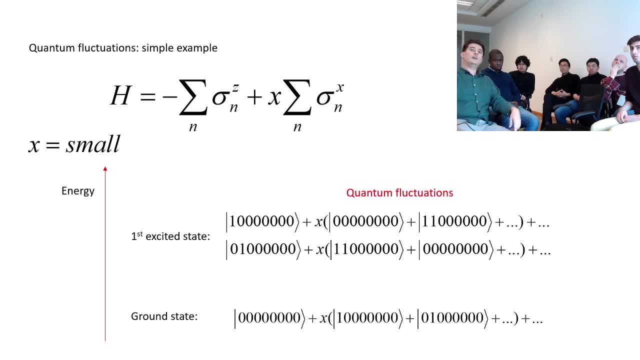 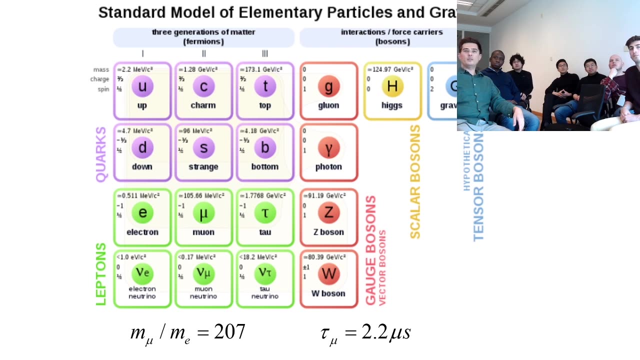 the muon or an electron that's like floating around, would be like one of these excited states and the fact that there's like extra terms. there are these sort of quantum fluctuations. Experiments that they're doing now are on the muon, which is like one of these fundamental particles. 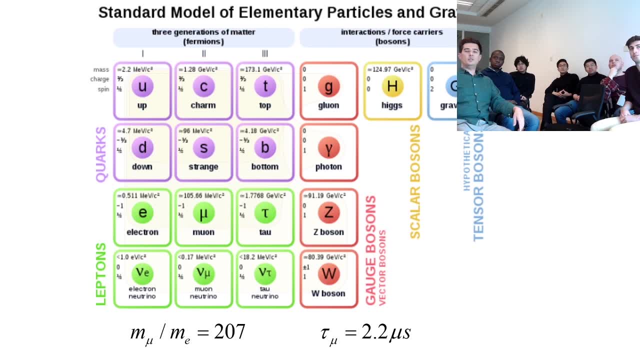 and so the electron is. you know, that's what we talked about. it was done in, you know, 1948. but the muon people are doing more experiments on and it's interesting because this has like a heavier mass and so the heavier the mass it actually includes, like, more and more like. 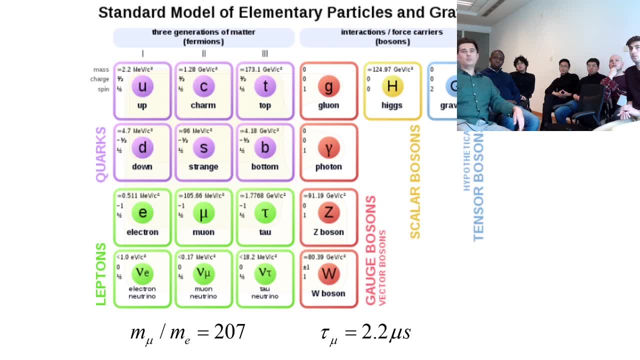 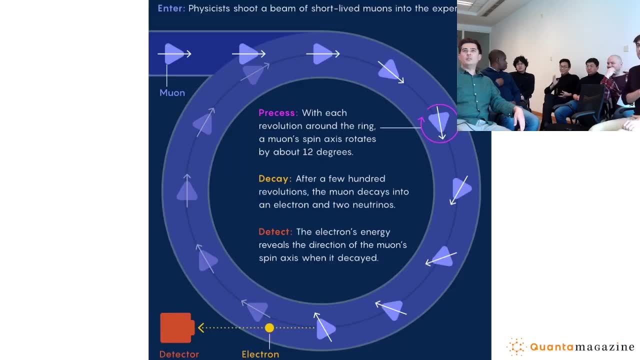 complicated effects that are going on. So it's a very interesting experiment. There's a lot of stuff that might arise from like QCD and other effects which you don't really see in the electrons. The way that they do this experiment is like they you know they shoot the muon into this. 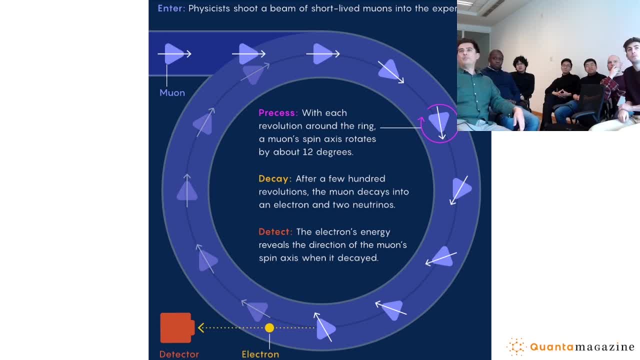 ring it goes around and the spin of the muon sort of precesses and and remember you know this is measuring basically the response of, like the, the spin to a magnetic field. so you know how much it precesses, is sort of you know how much of the spin of the muon is going to go into the magnetic field. 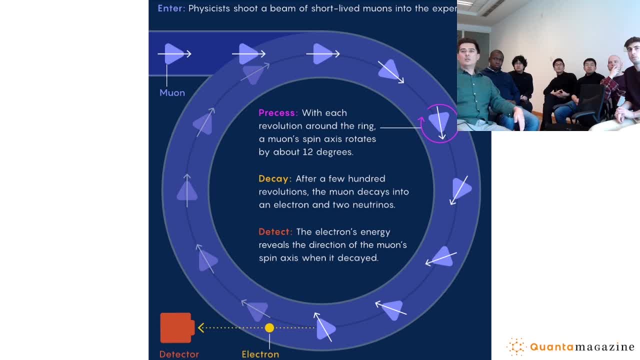 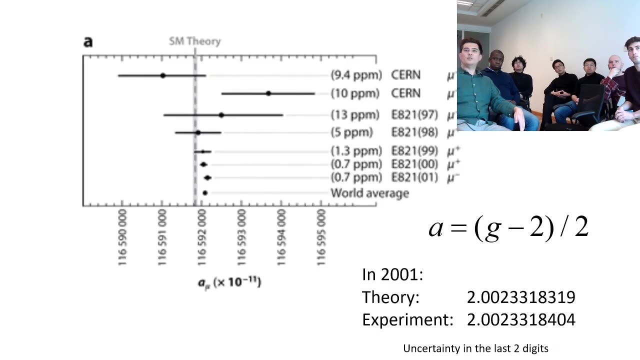 What you are trying to measure and then eventually you measure the amount of precession after it converts or decays into an electron, into a detector. So people already knew that in 2001 that it was looking a bit suspicious. that you know, theory was a bit different to experiment. so there's the theory in the experiment calculation. 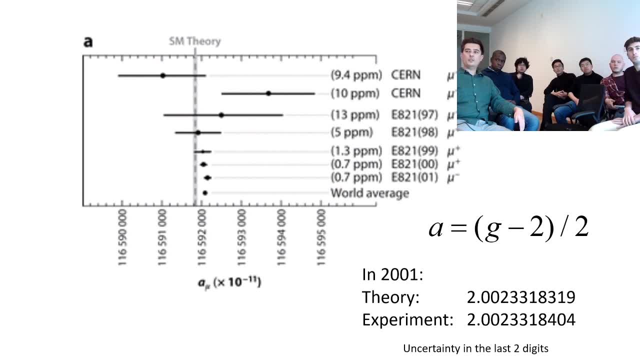 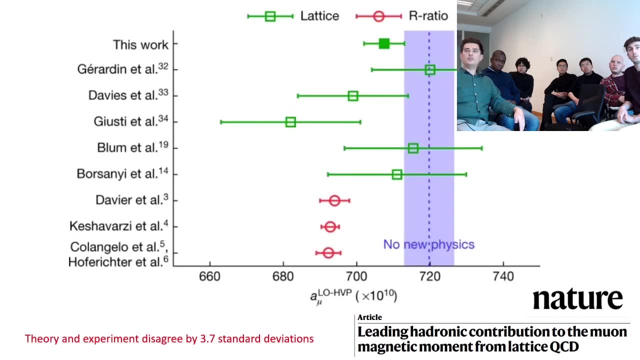 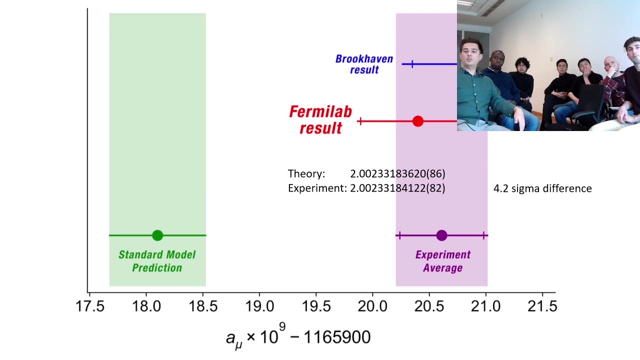 and you can see like there's a small difference in like the eighth decimal place. What the next generation of experiments are doing now is basically to basically come, you know, basically make a much more precise prediction. So this a thing is just defined over here, so it's. 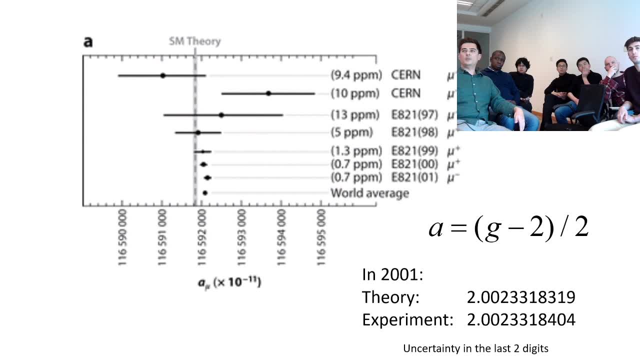 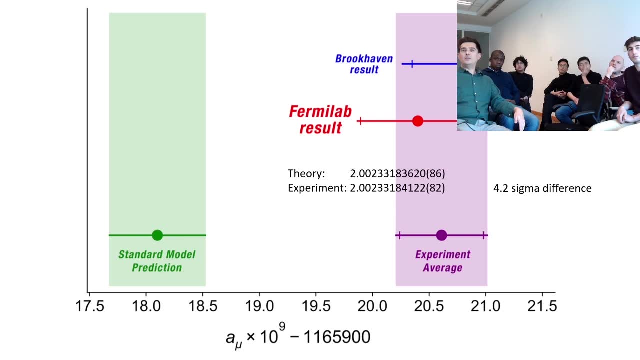 just like the difference from two. so you know, you subtract two from g and then, okay, divide by two, And so these are the latest results. so, basically, the results are still showing some quite a big difference to the standard model prediction so-called. well, so it's 4.2 standard. 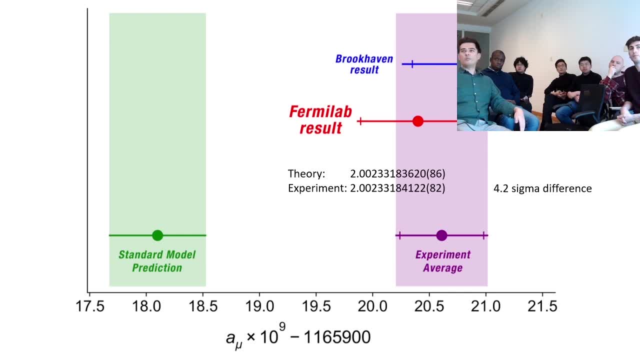 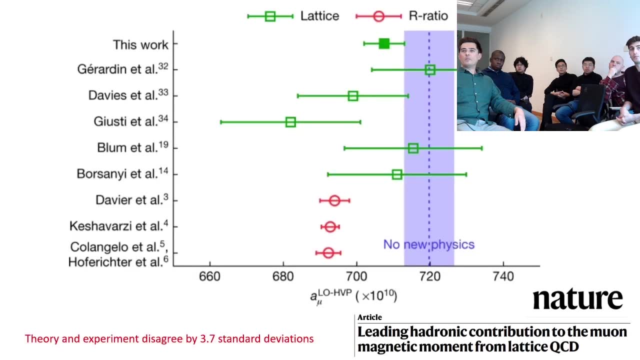 deviations different, which is kind of still quite, quite a lot. And then there's some latest paper that's come out now that's showing actually that maybe it's not quite so big, but then there's still some some difference. and so all these are different theory works, like the green and the red are all the different theory. 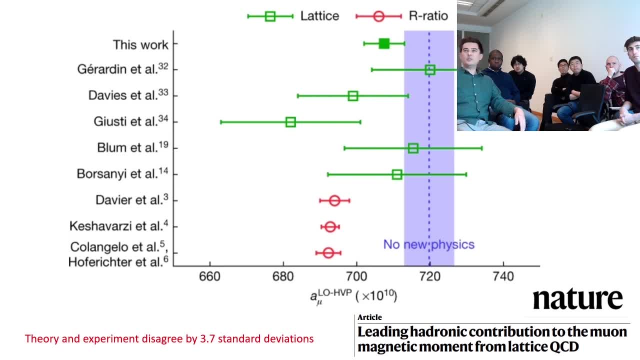 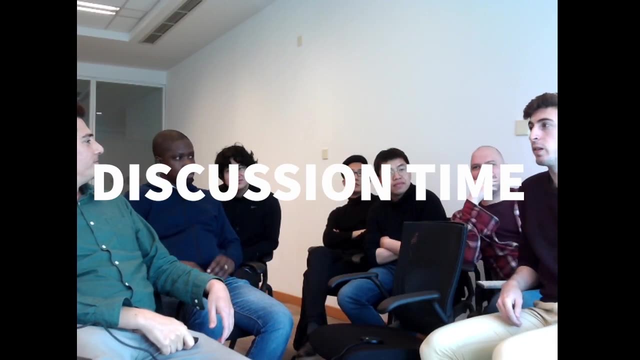 kind of approaches. so there's lots of different theory calculations going on to calculate this, but I think there's still a kind of consensus That there's difference to the experiment. so that's it. So even with the new nature paper, that still doesn't rule out the possibility that it's different. 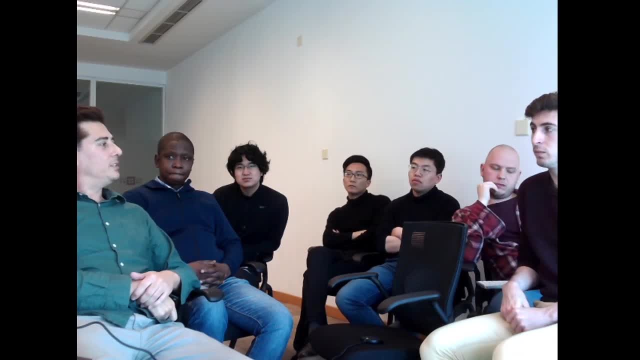 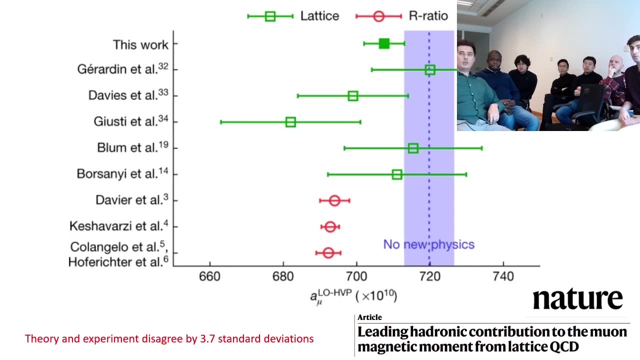 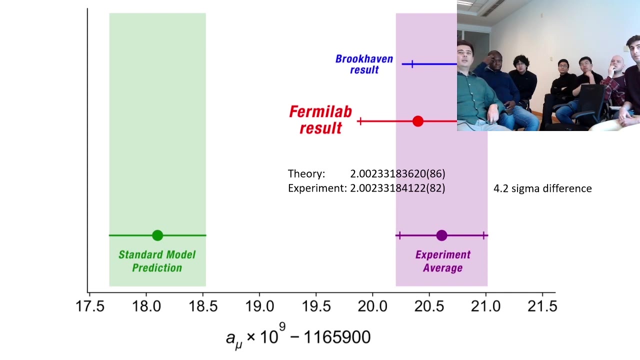 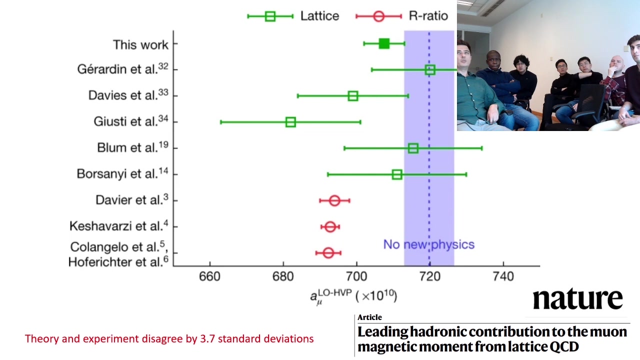 Seems like, yeah, so they in the paper, they say 3.7 standard deviations, yeah, and actually I don't know the difference to of this, well, of all these approaches to what was planned over here. So this is the Fermilab- you know, This is the Fermilab announcement- and they said 4.2 sigma. so I think there is some, you know, different sort of theoretical. 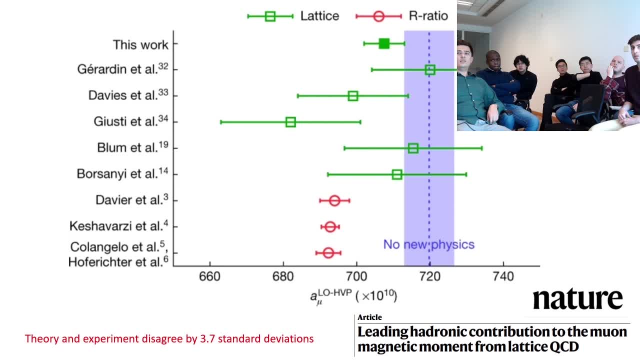 techniques, Ways to calculate. Yeah, like, I think particularly so. the title of this paper is, like you know, it's the, so it's the corrections due to lattice QCD, right? so there's some like QCD effects which are included in in these works which maybe you know. 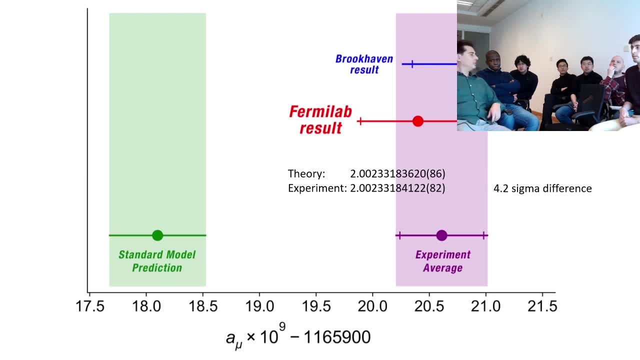 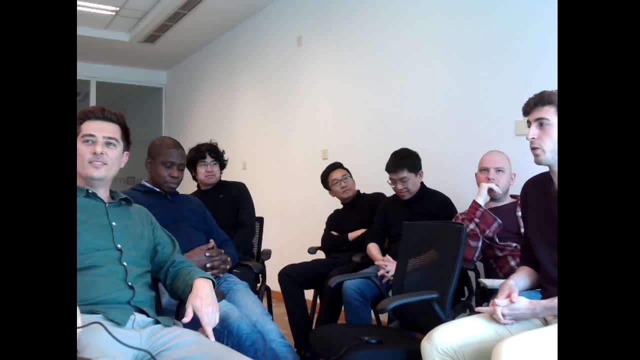 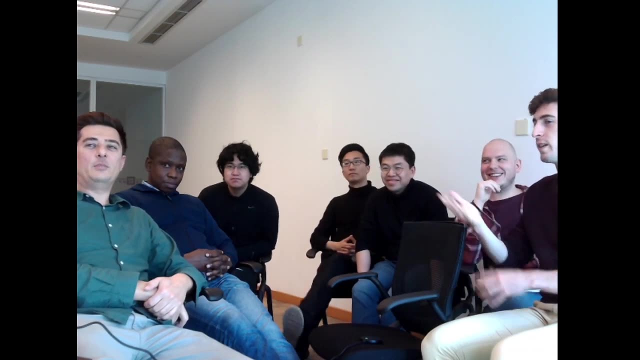 The 4.2 sigma is maybe, I don't know- it's only partially included or it's using a different technique, or something like that. yeah, So what would this result mean for the standard model That it's? you know? I guess that it's. why. is it something? something missing, right? yeah? 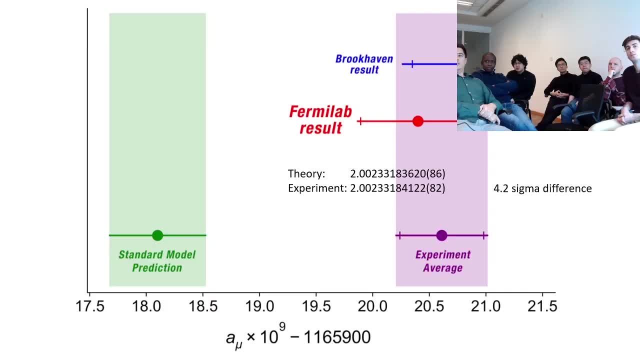 So that's what's so exciting, right? yeah, So, and Fermilab is saying that in the next round of iteration, maybe they are their standard deviation, might you know? they're much more precise, so the error will reduce more. Yeah, that's, that's the idea. to get this down even further. yeah. 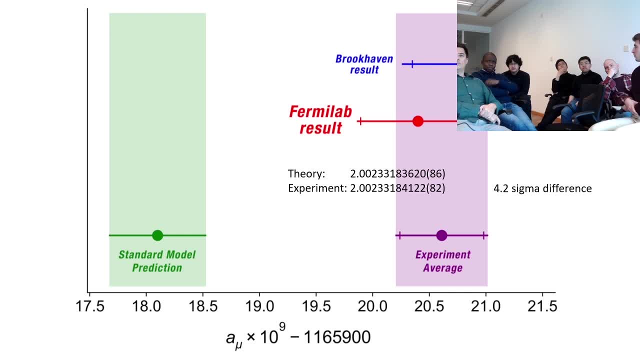 So, but even at that, I don't think it makes it correct. right, because the standard model is around 18. right, and this one is on the other side, 20.. Which one corrects the experiment? No, no, the standard model prediction is what I'm saying. yeah, the experiment seems to be within the 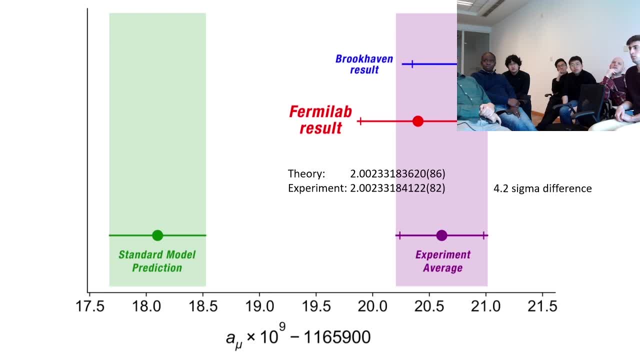 same, maybe the same error margin, because if you look at the lower end of Brookheaven result, I think it covers the average average experiment and even the Fermilab result. you know, yeah, the location of the red dot. so I think the experiment tool results are within the 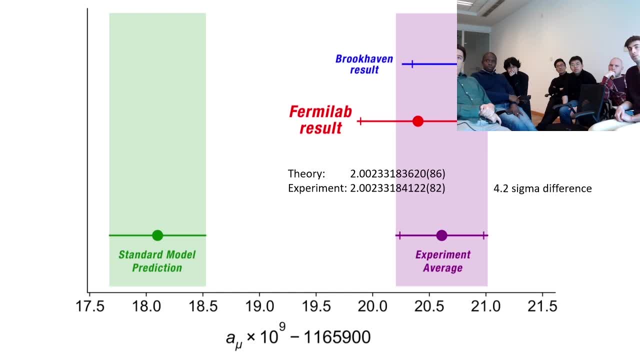 same error margin, but the standard model is really off. well, it's not off, I mean. well, yeah, I mean it is off. of course, yes, but it's like you know. so there's some. you know there's basically theory and experiment, right? yeah, so you know there's either something wrong with the theory. 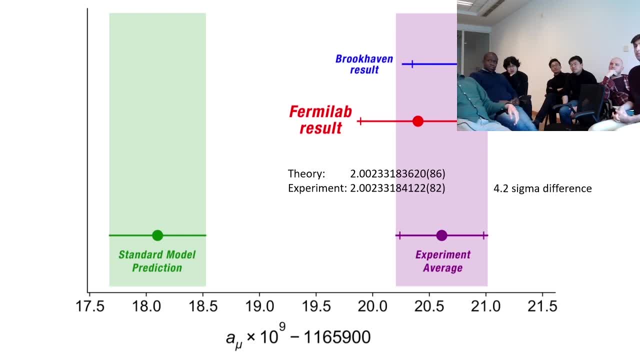 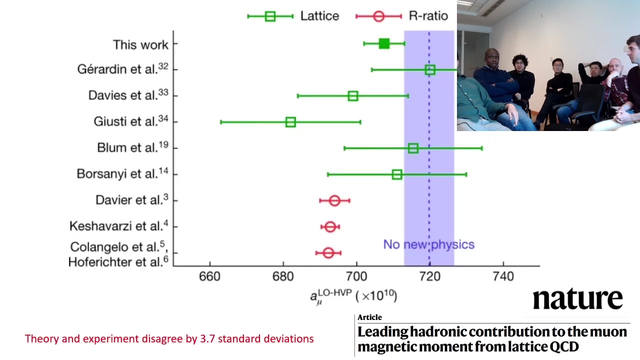 something missing in the theory? okay, yeah, or of course the experiment could be wrong, but of course we never doubt the experimentalist and mental is always right. yeah, or both are wrong. yes, yeah, yeah. but these QCD calculations, quantum chromodynamics, yeah, the lattice gauge simulations, what exactly do they really do they include more parameters or more theories? they? 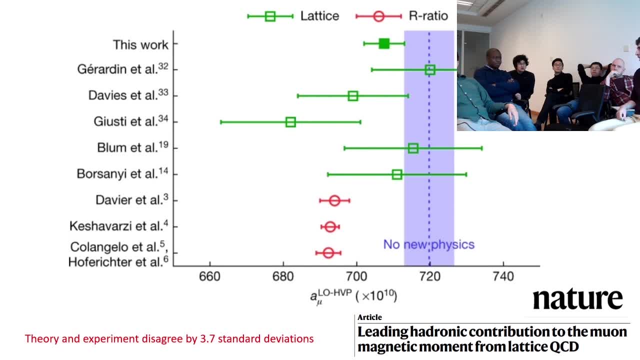 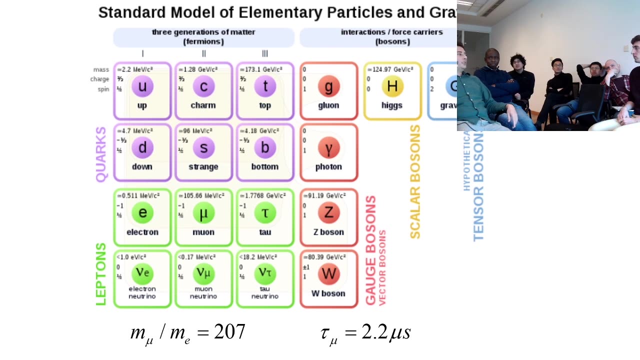 throw in more things or they remove. this. is it just adding more complex Feynman diagrams? you just like add more and more branched out. yeah, I'm not sure, because you know properly, read the paper, but I imagine from you know the thing with QCD is that it's